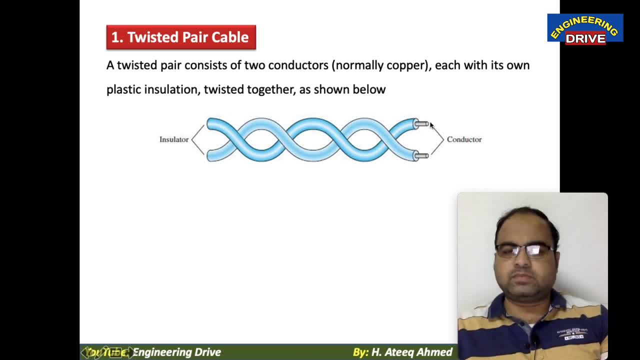 What we call this one Conductor. And what is the material which is used to design this conductor? It is a copper. And above this conductor, there is one more layer. We call this layer as insulator, What we call this one Insulator. Is it okay? Now, one of the 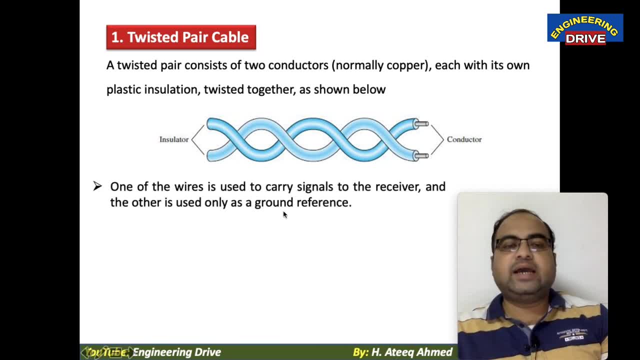 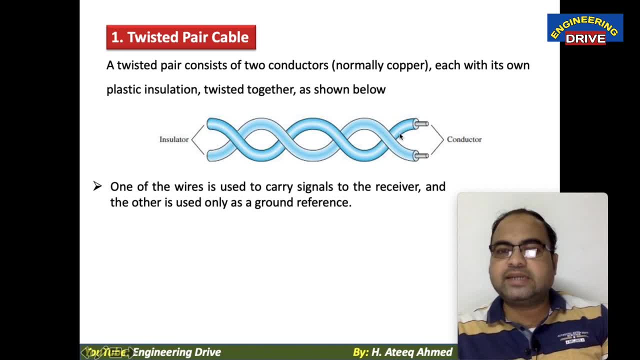 wires. one wire is used to carry the signals. Let us say, this wire will carry the signal. What about the second wire? Second wire will be used as a ground reference. So this is very, very important point in Twisted Pair. Next, dear students, in addition to the signals, 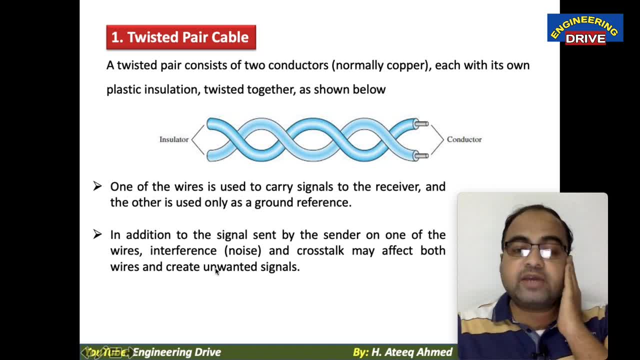 sent by the sender on one of the wires. interference and cross talk may affect both wires and create unwanted signals, So there is a problem in this. So what would be the problem here? Here we have a wire in this wire. This wire will be used as a ground reference and this wire 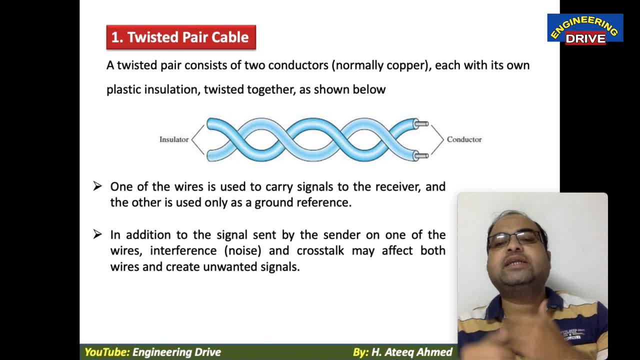 you know, there is a chance that interference or any type of cross talk may happen. so, in order to overcome or reduce this problem, what we can do, instead of keeping the voids in a normal way, we can make them twisted. so this is the point which says this explanation: by twisting the beds. a. 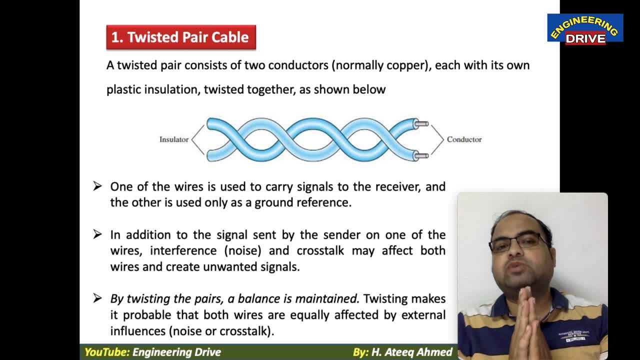 balance is maintained. this is very important. now you people can ask one question, sir, why we are twisting the voids are simply, we can keep the voids straight. if we keep the voids straight, there is a problem of interference, there is a problem of noise, there is a problem of cross talk in order, 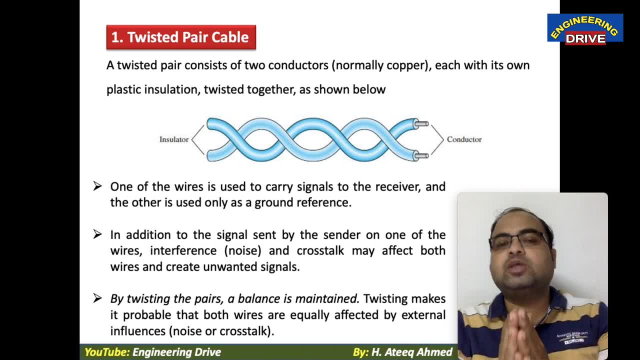 to overcome that problem. we need to twist the beds in order to maintain the balance. so twisting makes it probable that both voids are equally affected by external influences that can be noise or cross talk. so this is the reason why we twist this pair of cables, is it okay? next continuation: the most 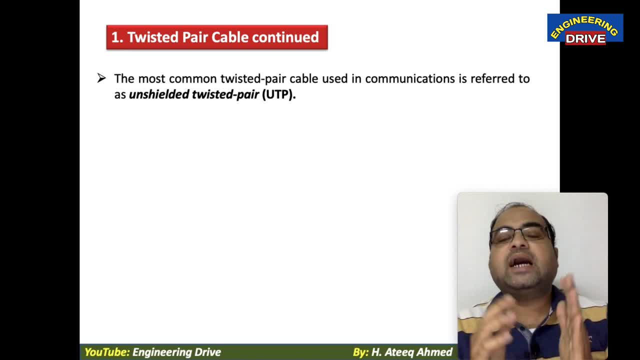 common twisted pair cable used in communications is referred to as unshielded twisted pair, so this is the cable which is used in most of the communication system. so it is known as utp unshielded twisted pair. and there is one more category in this: ibm has also produced a version of twisted pair cable for its use. 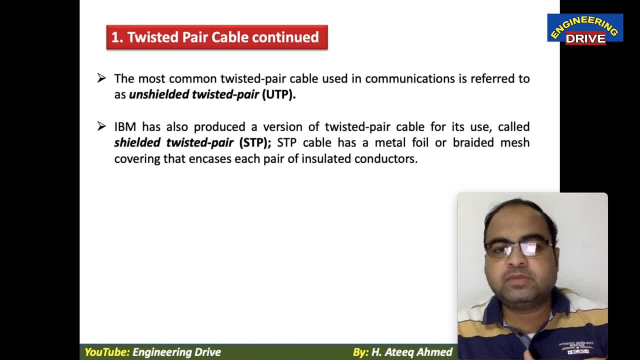 called shielded twisted pair. that is stp. stp cable has a metal foil or braided mesh covering that encases each pair of insulated conductors. now you can see, dear students, in twisted pair we are having two types: unshielded twisted pair and shielded twisted pair. you can see. 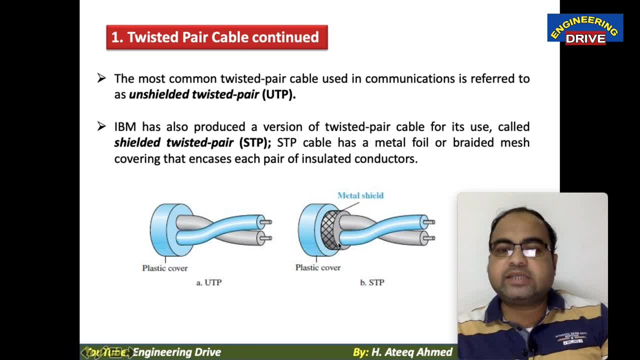 there is only one difference between them. what is the difference? extra metal shield is available here in shielded twisted pair. shielded meaning. meaning is more protection. we are providing here, how we are providing more protection to this cable. we are providing more protection to this cable with. 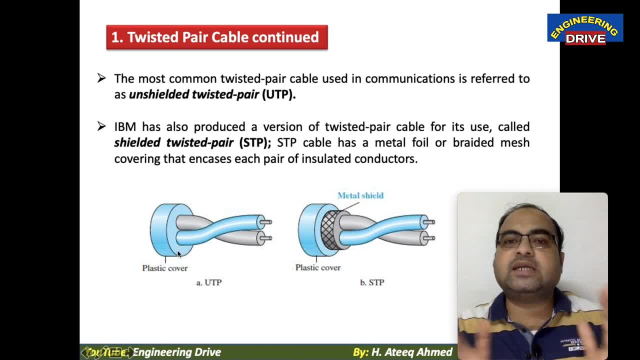 the help of one extra metal shield. you can see here, in unshielded twisted pair, there is no extra metal shield, whereas in shielded twisted pair, this extra metal shield is available. you know what is the use of this extra metal sheet? the main purpose is to protect this wire from any type of interference or 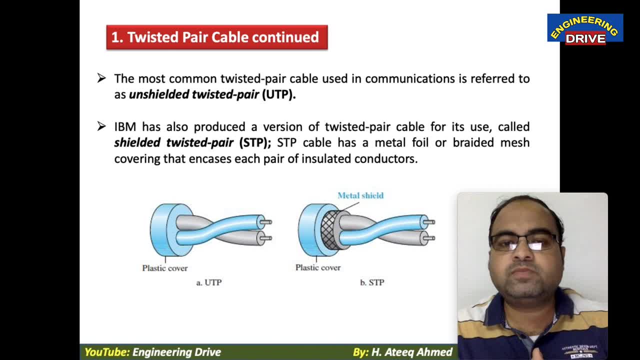 unwanted interference. is it clear? this is how a twisted pair cable looks, and these are the two subtypes in this. next, coming to the second tool names is then twister. it is a t 관련 one. when it comes to to this external power supply, we are going to talk for the first time about how a sister power supply 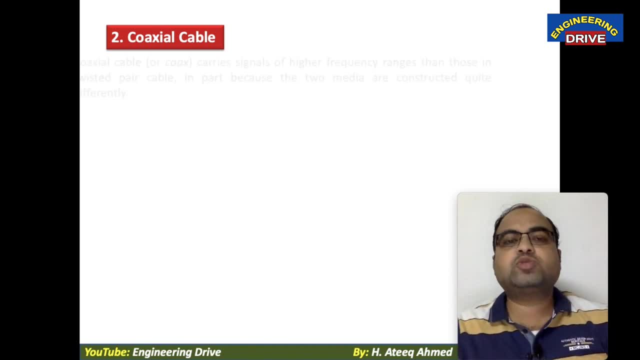 is a chip and it is a highly torqued, soldable chip which is a durable, used for次 design which processes guided media coaxial cable. okay, what is coaxial cable? coaxial cable, or it is simply known as quacks, carry signals of higher frequency ranges than those in twisted pair cable, in part because 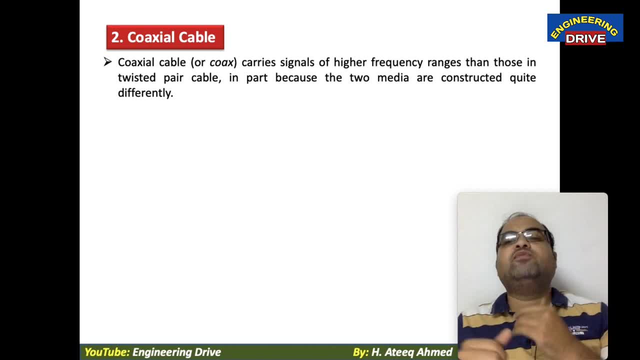 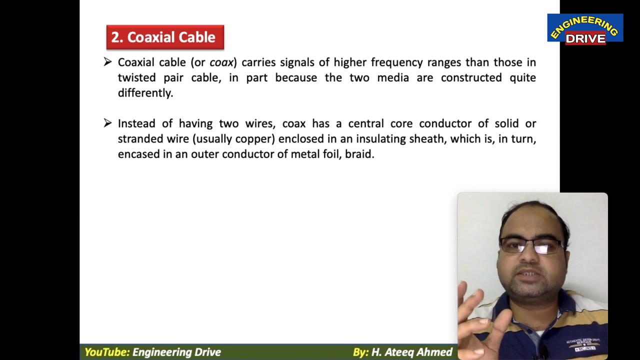 the two media are constructed quite differently. now, if you want to transfer or carry the signals, if a wire need to carry the signals of higher frequencies, then twisted pair cable will not work, so we need to make use of this coaxial cable instead of having two wires. coax has a central. 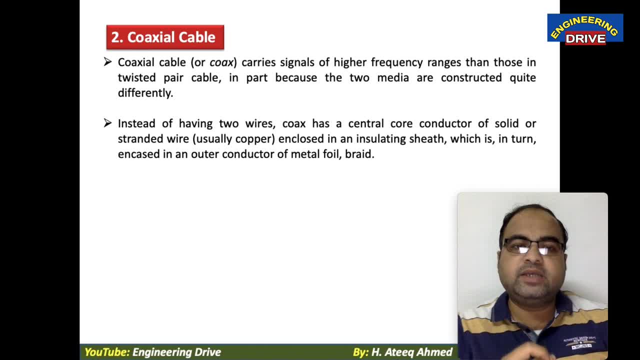 core conductor of solid or stranded wire, usually copper, enclosed in an insulating sheath which is in turn encased in an outer conductor of metal foil braid. so here what happened. instead of having two equal wires, what happened? the wires are arranged in a layer fashion. here how the wires: 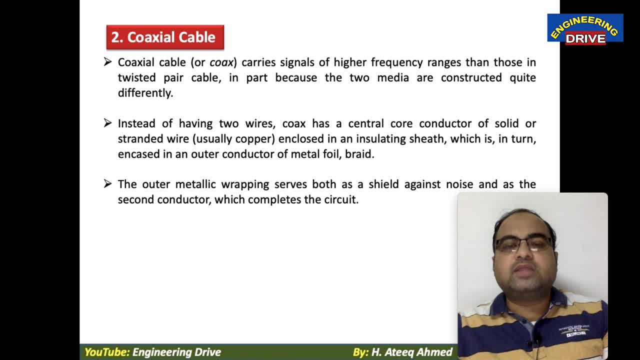 are arranged in a layer fashion, so we need to make use of this coaxial cable instead of having two wires. so we need to make use of this coaxial cable instead of having two wires. so we need to make use of this coaxial cable. let me show you the outer. metallic wrapping serves both as a shield against noise and as the second. 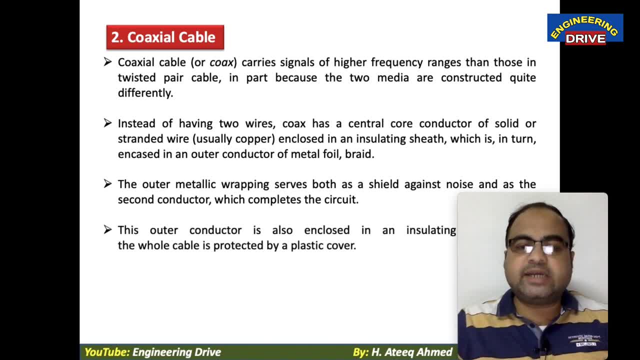 conductor which completes the circuit. this outer conductor is also enclosed in an insulating. the whole cable is protected by a plastic cover. now, dear students, this is the points which i have explained. you can understand now with the help of this diagram. you can see here, two conductors are there. this is this conductor is an. 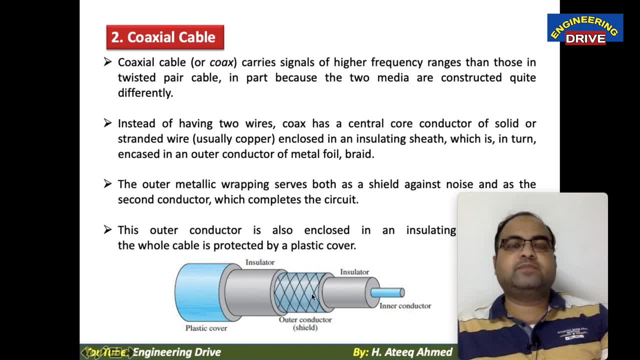 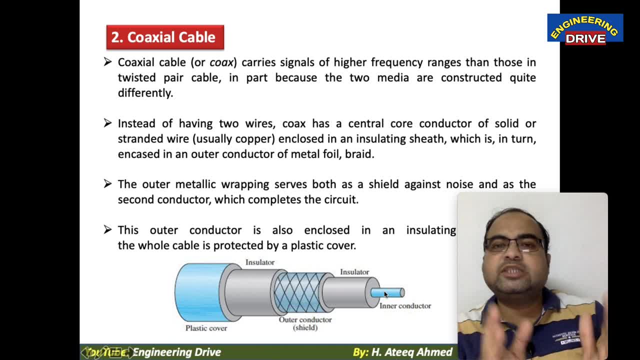 conductor. why we are calling this conductor? as inner conductor, it is present inside. why we are calling this outer conductor? because it is outside the inner conductor. now, both this inner conductor and outer conductor has been covered with insulators, so you can see here. so, inner conductor, there is insulator to protect the inner conductor and to protect the outer conductor, there is one. 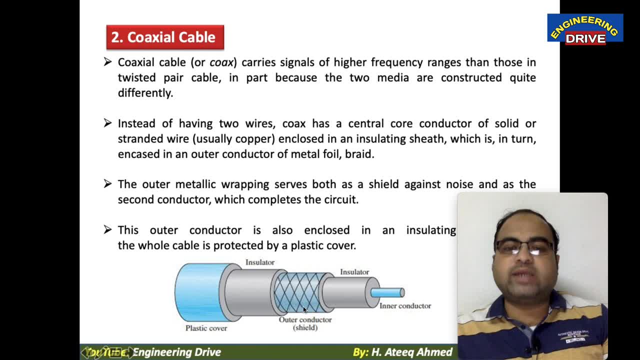 more insulator. now, to cover this entire coaxial cable, there is a plastic cover for added safety. now you can see the main difference between the twisted pair cable and coaxial cable is. in twisted pair cable the both the wires have been twisted equally, whereas in coaxial cable 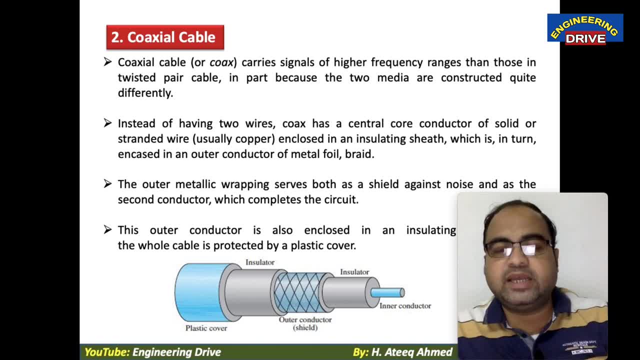 these two conductors have been aligned in a layered fashion, okay, so that it can have more protection from the interference. so coaxial cable provides better transmission of data compared to the twisted pair cable. in simple, short summary, is it right now the third category of cable and 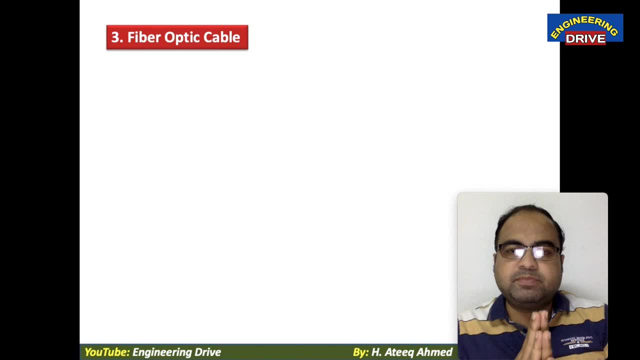 which is one of the best way or best transmission media to transmit the data is the fiber optic cable. so this is the first category of cable and which is one of the best way or best transmission. so this is the third guided media. a fiber optic cable is made of glass or plastic and 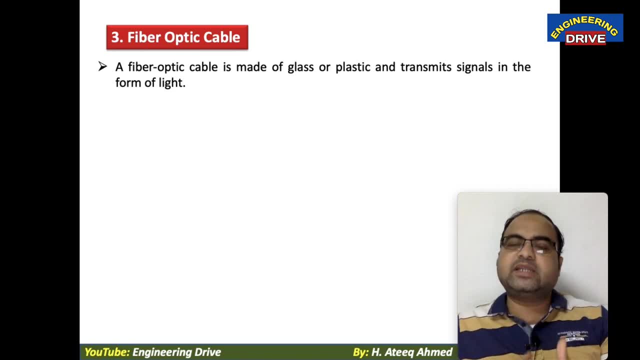 transmits signals in the form of light. now, if you want to transmit the signals in the form of light, twisted pair cable will not work. next, coaxial cable also will not work. then we need to have only one option, that is, the fiber optic cable. optical fibers use. 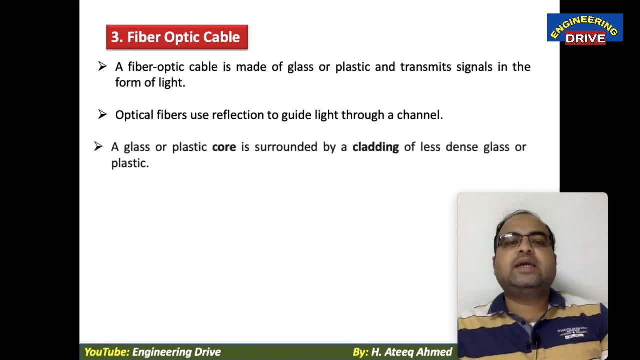 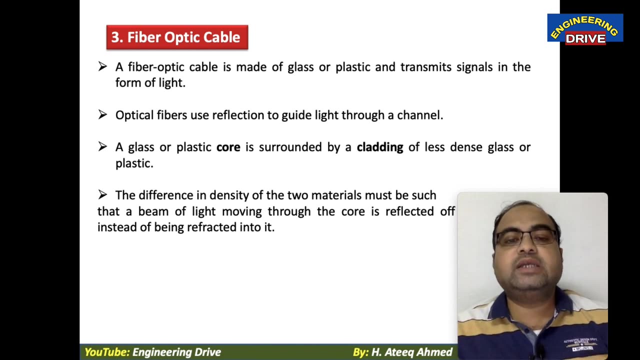 reflection. to guide light through a channel, a glass or plastic core is surrounded by cladding, dense glass or plastic. the difference in density of the two materials must be such that a beam of light moving through the core is reflected off instead of being refracted into it. now, when we 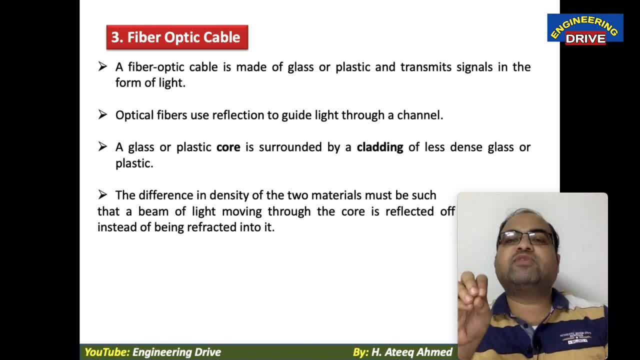 are talking about fiber optic cable. it will work on the concept of reflection of light. so the beam of light which is traveling in the optical fiber in the fiber optic cable will perform reflection. so because of that reflection, that data will be transmitted directly from sender to the receiver. 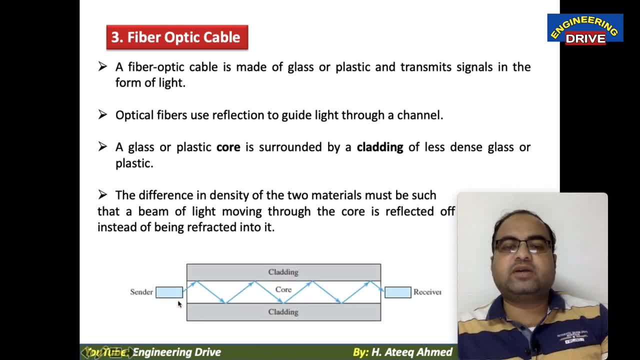 now you can see here. this is the diagrammatic explanation of the fiber optic cable. this is the core where the data will be transmitted, the light will be transmitted, and here the left side is the sender and here it is the receiver. now, to protect this core, a cladding layer has been added, so which? 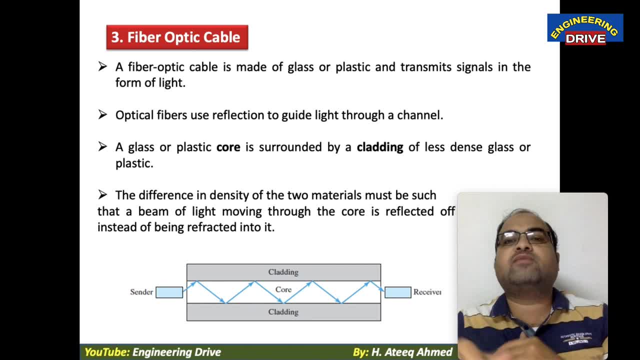 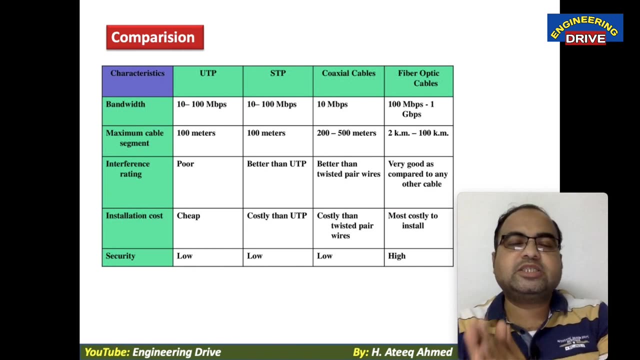 makes the light to be inside the cable only, instead of going outside the cable. this is what the work of cladding. so, dear students, this is how the fiber optic cable works. now the main question, sir: which one should be preferred and what are the advantages and disadvantages of these three guided medias? so this is a table which which I am going to show. 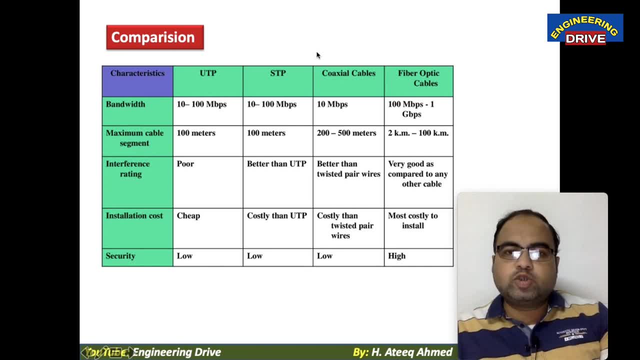 you the difference in characteristics of these three categories. so for twisted pair, we know that there are two types. what are those? unshielded twisted pair, shielded twisted pair. and then the second guided media is coaxial cables and the third guided media is fiber optic cables. so if 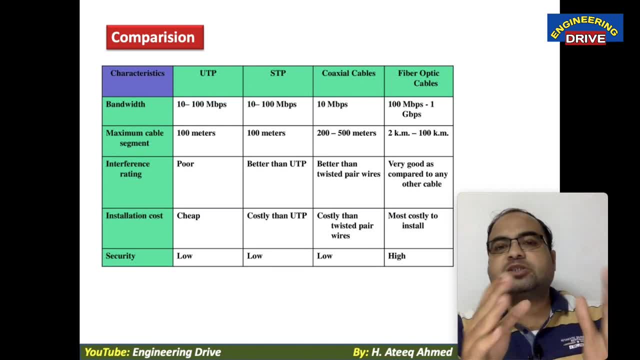 you concentrate on this table, you will understand 90 percent of the concept. anyhow, a small summary I am going to show you now, before I am going to close this today's session. now, in terms of bandwidth, the highest bandwidth will be in fiber optic cables only, which ranges between 100 megabits.